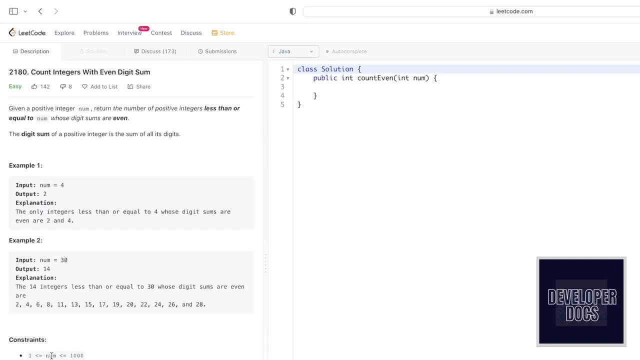 are even numbers. those 14 numbers are equal to digit 68, which is the sum of the digits in 4. are these? and the value of num will be within 1 and 1000, so the maximum range will be 1000.. So this is a fairly easy problem. First we'll write a helper function which will return the 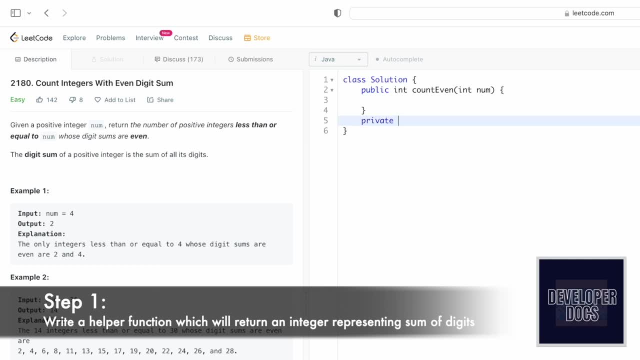 digit sum. Since this will return the sum, it is going to be an integer, which is the return type. I'm going to name it sum of digits and pass an integer n. Now let's create a variable sum which will store the sum of all the digits present in n. So let's use a while loop to calculate the sum. 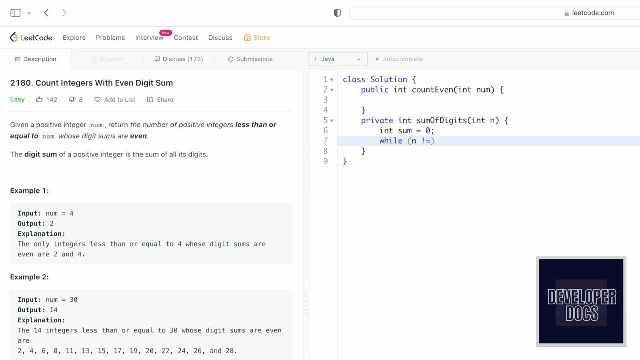 and this while loop will run until n is equal to 0. So until n becomes 0, this while loop will run. Let's start by extracting the digits from the last in n, Save it inside a variable digit and extract the last digit using the modulus operator. Now we 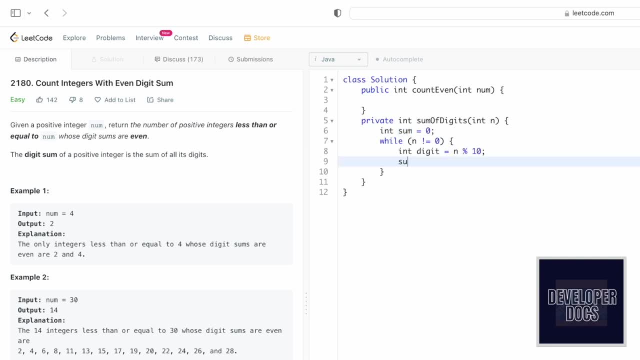 have the last digit, Let us add it into sum and repeat the process again. Sum plus is equal to digit. Sum is initially zero and now we keep adding the digit from the last. Now, before starting the next one, Let's create a variable which will store all the digits present in n. Let's create a variable. 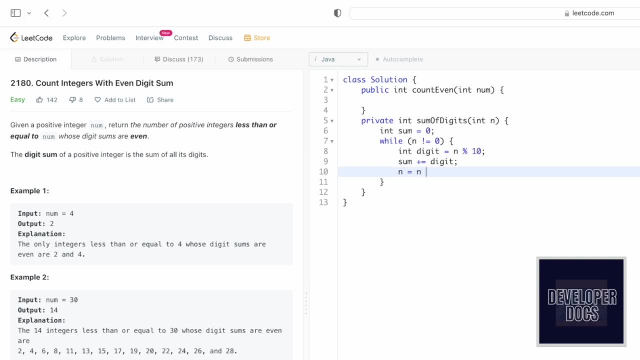 iteration. let us decrease the size of n by removing the last digit, and now you have to continue until n becomes 0 and finally, after the while loop ends, you will get the sum inside this variable so you can return it. So return sum. Now we have a helper function which will give us the 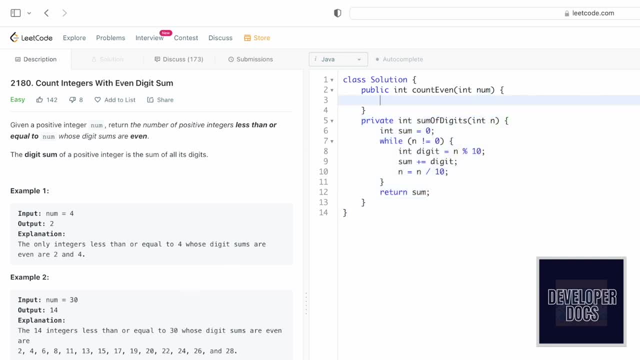 sum of digits and we have the range. So let's start the range from 1 until num. So for n, i is equal to 1 and i is less than or equal to num, and in each iteration i will be incremented by 1.. 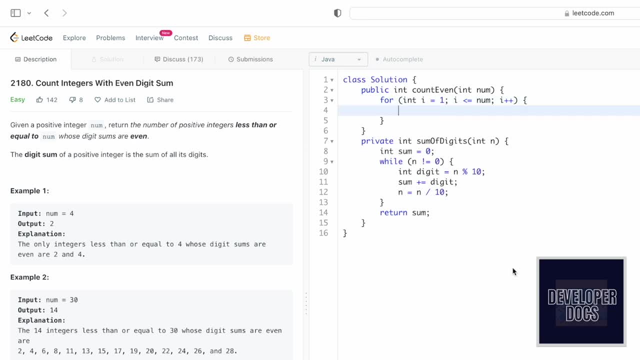 Now we have to check if the sum of digits in i is an even number. If let's call the helper function which we have written, sum of digits of i is an even number. So when you divide it by 2 you have to get a remainder of 0. If that is the case, you increment the count, So you increment a variable. 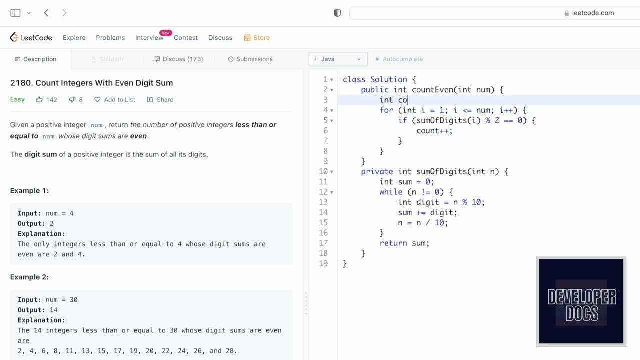 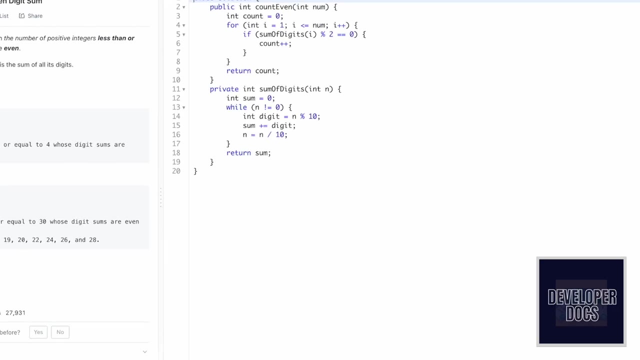 count. First, let's initialize that variable, which is initially 0, and whenever this condition satisfies, you, increment the count and finally you can return this variable count, which will be our result, counting the number of integers within num whose digit sum is an even number. Now let's try to run. 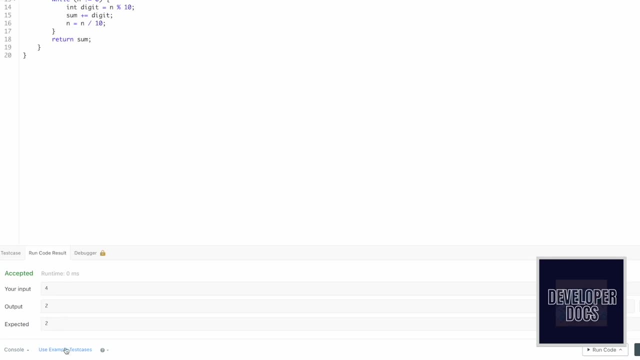 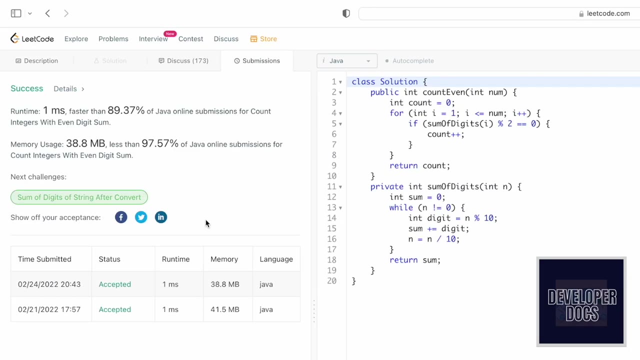 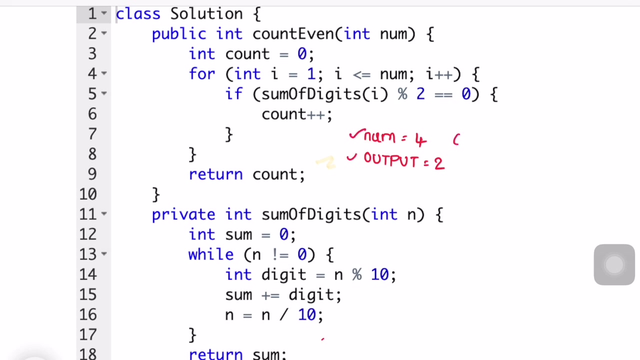 the code. We're getting the expected output. Let's test for all the test cases. It is accepted. Let's submit the solution. There you have it. Our solution has been accepted. So let's take this example. We have a num called 4 and the output is 2, because the two numbers are 2, 4.. So let's see how this. 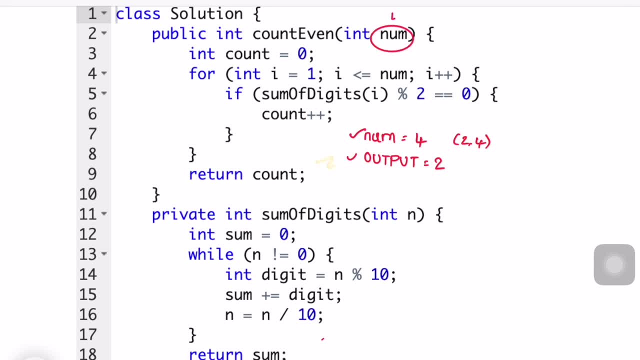 program will work Now. num is having the value 4.. So this for loop will run from 1 to 4.. We're calling the function sum of digits, where i is equal to 1.. So n is first 1 and the sum of the digits in 1 is. 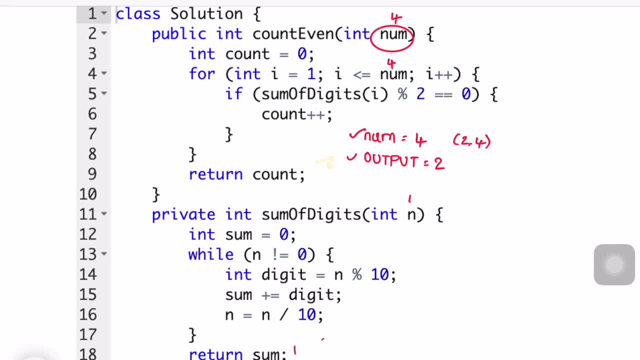 equal to 1.. So this will return 1.. So 1% 2 is equal to 0.. It won't return 0. It will return 1.. So count is still 1.. So we have a num called 4 and the output is 2, because the two numbers are 2, 4.. So let's. 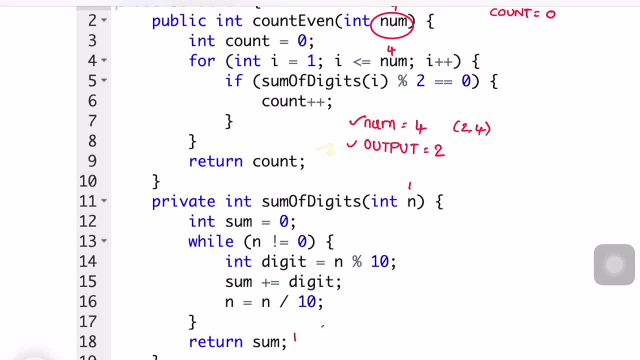 blindlyApply this. Next iteration we have 2.. For counting only let's run the operation with 2 towards 3.. So count will be 1, because no num will return 0. So last time Teaching machine here is: paste 3 plusIT, 파일3 F, else power into 0. So next iteration we have 2. So i will be, i equals. 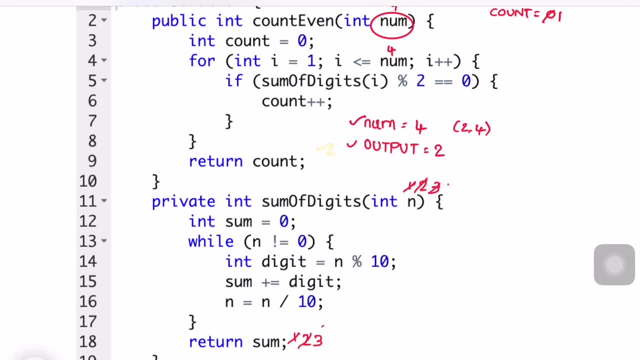 1.. And understanding that we have 3,, 4 and 0. So counting, even order, will not be as vertical understanding of this. So we're calling this function to four like 1, we're counting it and again, instead of 4, we're jelly like 1.. So this will return 0. So count will be equal, Shell 1.. 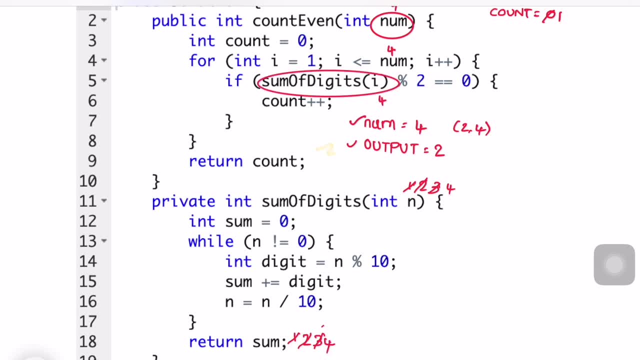 so this will return 4.. 4 modulus 2, yes, it returns 0, so count will be incremented, so count is equal to 2.. Next iteration: i is equal to 5, but this condition will fail, so it won't enter inside the for loop and count will be. 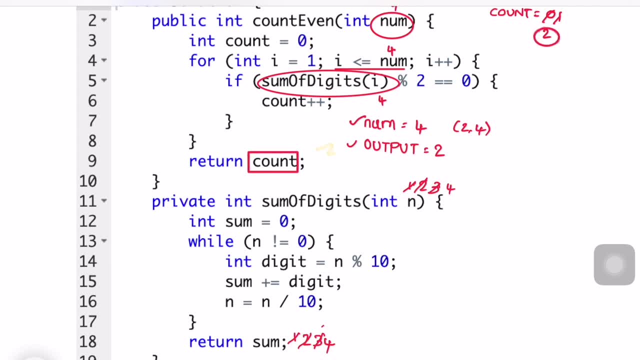 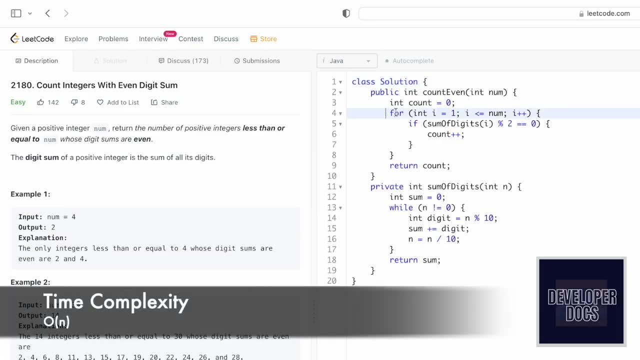 returned as the output. which is having the value equal to 2 will be returned as the output. Hence 2 is the output which we are getting for this question. The time complexity for this approach is O and the space complexity is O, That's. 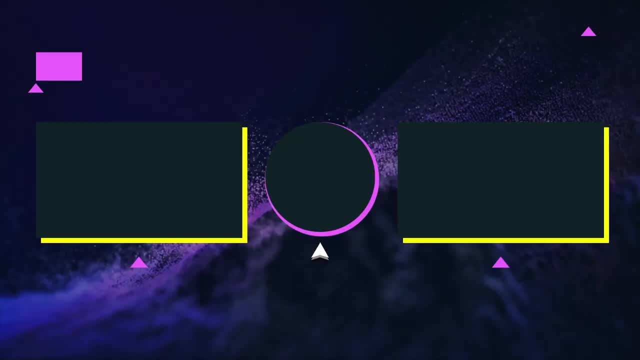 it guys. that's the end of the video. thank you for watching and I'll see you in the next one.